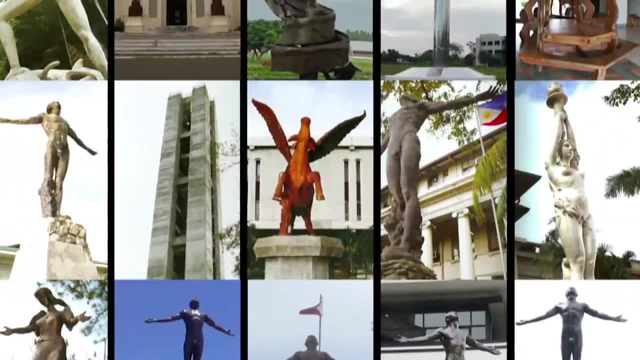 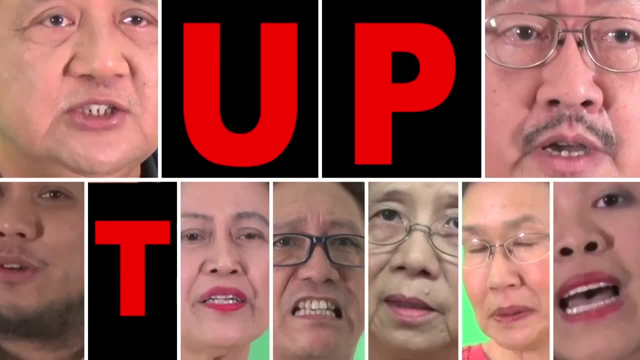 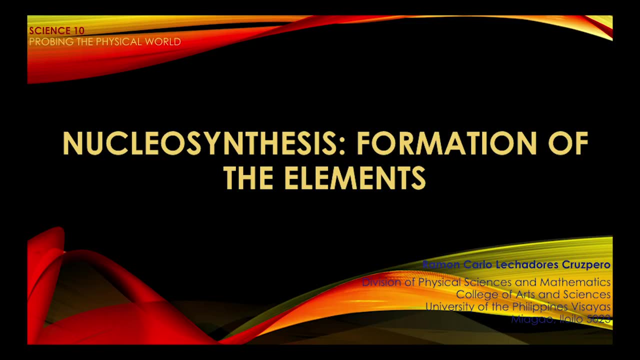 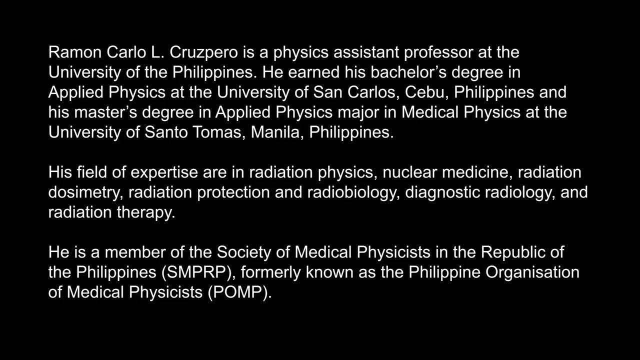 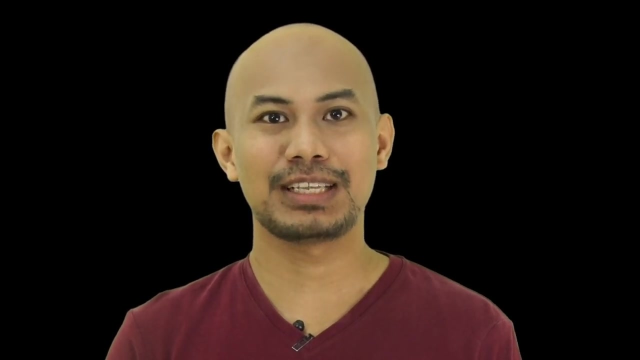 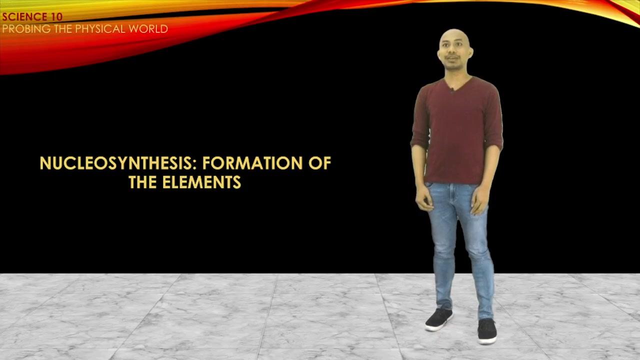 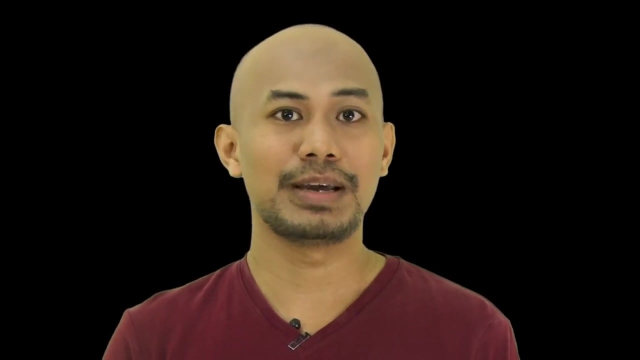 Thank you for watching. Thank you for watching Which element or elements were used in the creation of such spectacular colors. My takeaway in this kind of nerdy, or, shall we say, educational discussion is rooted from one key point: the chemical elements. But what are chemical elements? 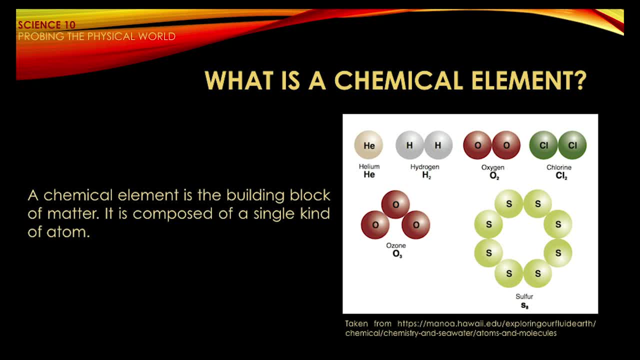 We have encountered this term in our chemistry class and defined it as the building blocks of matter. We also have known that a chemical element is composed entirely of one kind of atom. Now, where do these chemical elements really come from? How were they created? 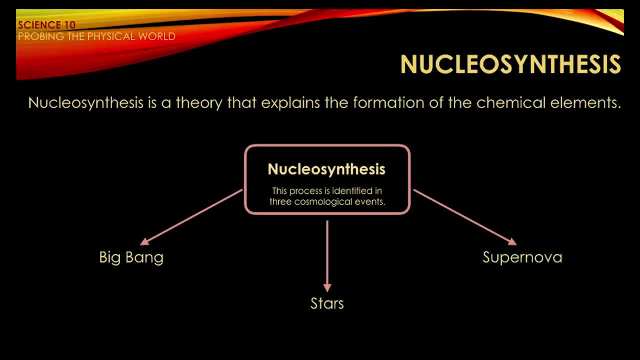 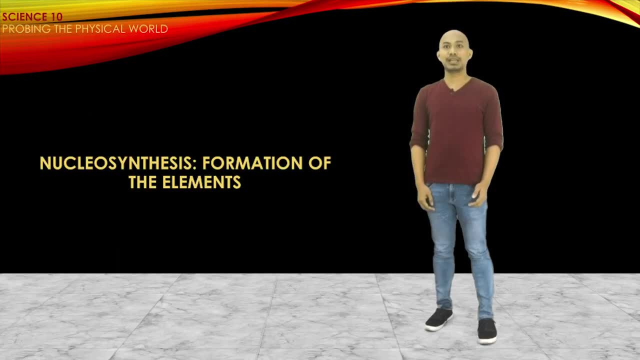 These questions are answered when we study nucleosynthesis. This is a theory which explains the formation of the chemical elements that we know today. In the storyline of the birth of the universe, there are three identified cosmological settings where these elements were believed to have been created. 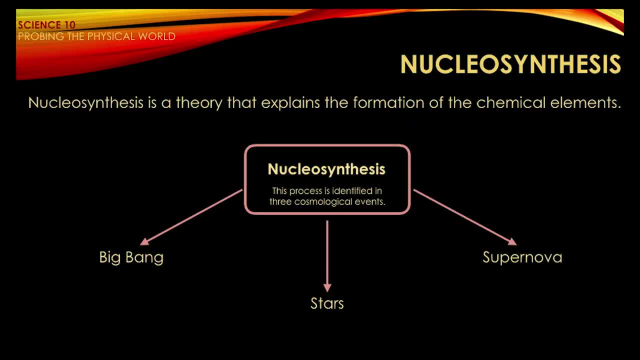 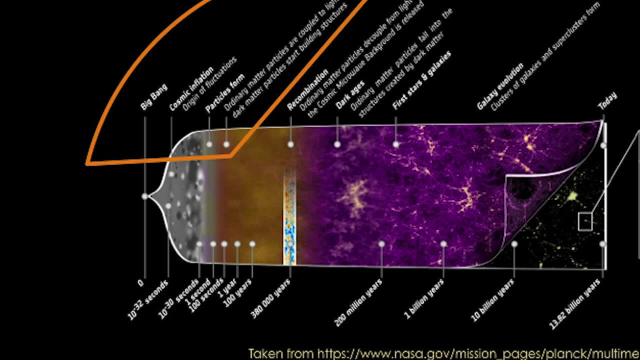 These are the Big Bang, the stars and the supernova In the early parts of the Big Bang timeline. as the temperature cooled down, the massive energy brought by the Big Bang created the fundamental particles such as the leptons and the quarks. 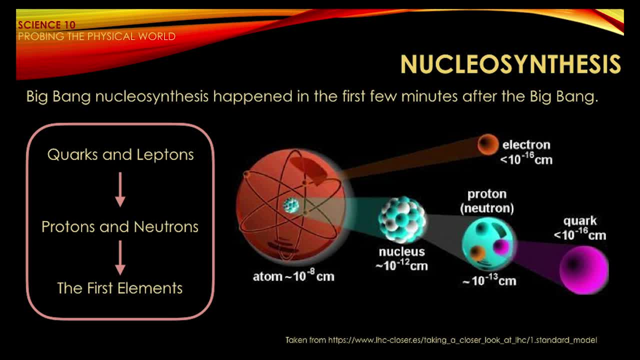 Due to the relatively high temperature, these newly created particles were moving so fast that a number of collisions among them happened, but they weren't able to combine As the temperature continued to decrease due to the expansion of the universe, these fundamental particles were able then to interact and combine to form the atomic particles, namely the neutrons and the protons. 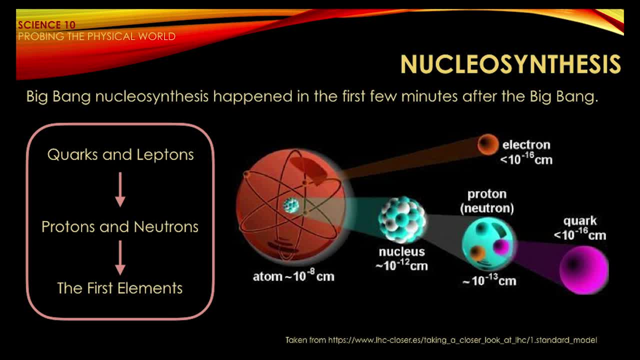 With a further continued decrease in temperature. these atomic particles interact with one another to form the first two elements in the universe: helium and hydrogen. There were some traces of lithium and beryllium formed due to the formation processes of the first elements. particularly in one of the formation processes. The first two elements were the helium and beryllium, but the early lithium and beryllium were unstable and they decayed into more stable elements, most likely helium-4, or the isotopes of the first two elements. 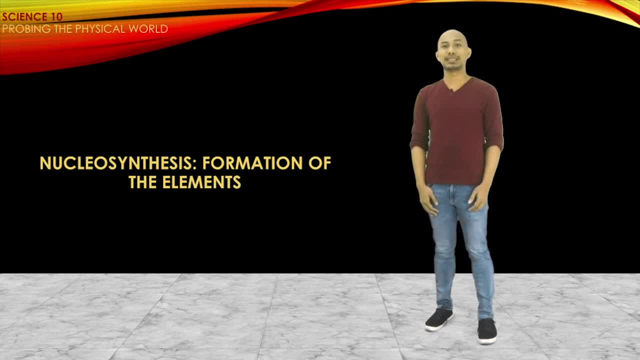 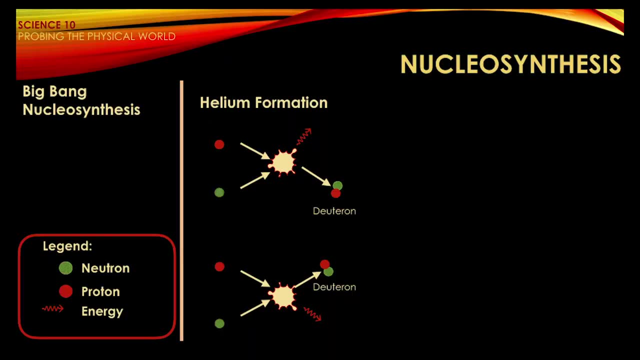 There are a number of processes in the formation of the helium element, but according to George Gamow, the formation process of helium-4 may take three steps, as shown in this illustration. The first step involves two separate interactions of a neutron and a proton, which each create a deuteron. 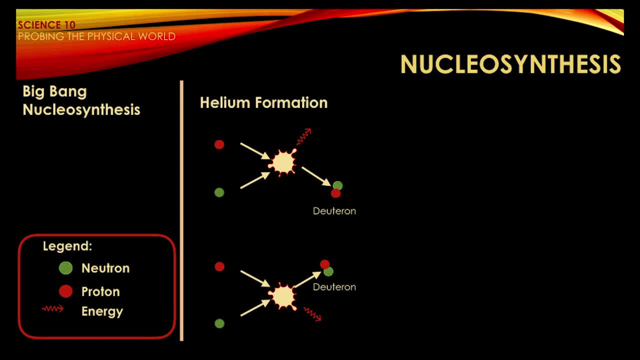 A deuteron composed of a neutron and proton is the nucleon of deuterium, an isotope of hydrogen. The second step involves the interaction of two deuterons, which results to an ejected neutron and the formation of helium-3 atom. 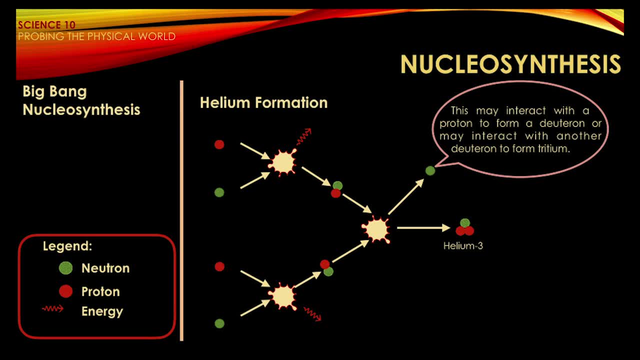 Helium-3 atom is an isotope of helium-4 and is considered as one of the most stable isotopes in the universe. On the other hand, the ejected neutron may interact with another proton to form another deuteron, or may interact with another deuteron to form a tritium, which is another isotope of hydrogen. 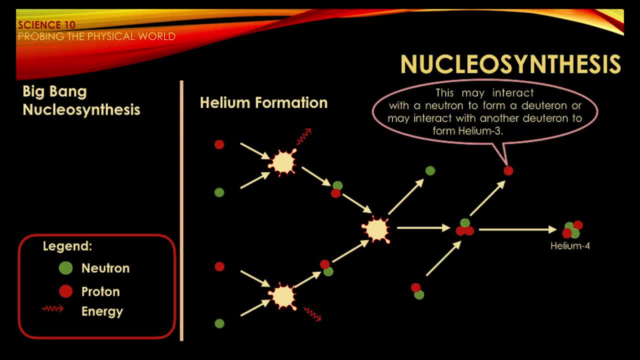 The third step is the interaction of helium-3 and a deuteron. This will result to the formation of helium-4, with two protons and two neutrons and an ejected proton. The ejected proton may interact with a neutron to form a deuteron or interact with another deuteron to form helium-3. 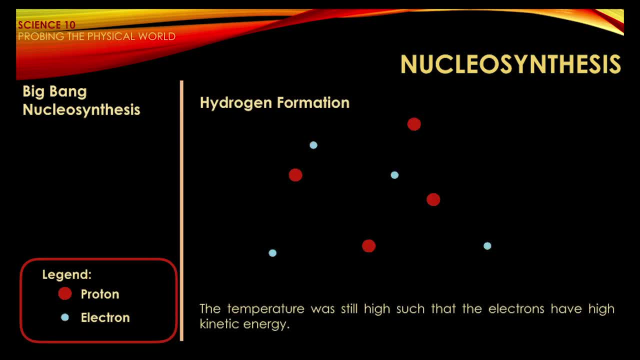 On the other hand, hydrogen was created when a proton attracts an electron to revolve around it. At first, there were only few hydrogen atoms created as the electrons were still moving fast due to the relatively high temperature. But as the temperature continued to decrease, these electrons gradually slowed down and a proton had a higher chance to attract an electron. 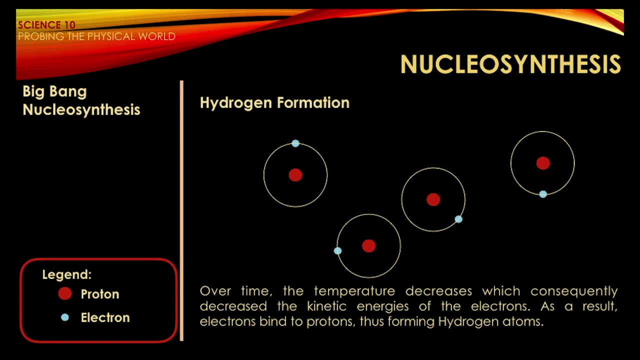 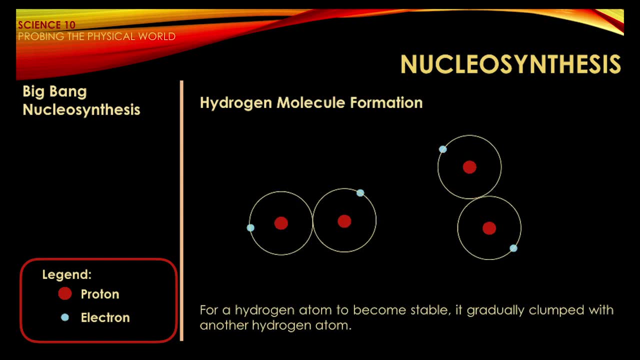 Because of the simplicity of this process. this is the reason why hydrogen is the most abundant element in the universe. For a hydrogen atom to become more stable, it attaches to another hydrogen atom, thus forming a hydrogen molecule. These hydrogen molecules, together with helium atoms, clump together to form molecular dense clouds, which are the main ingredients of the formation of stars. 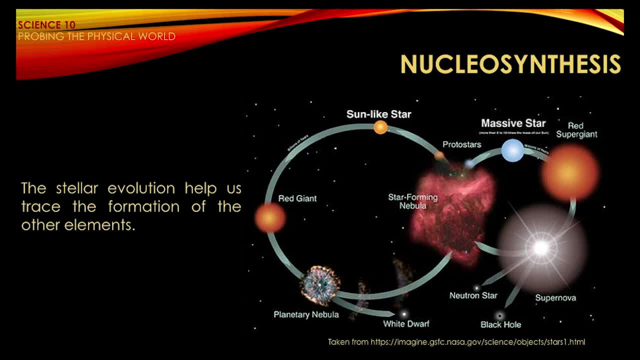 The stellar evolution helps us in tracing the formation of the other elements. The life of a star generally begins when a gravitational collapse of cool, dense molecular clouds happens. As these clouds collapse, they fragment into smaller regions which themselves contract to form stellar cores, the protostars. 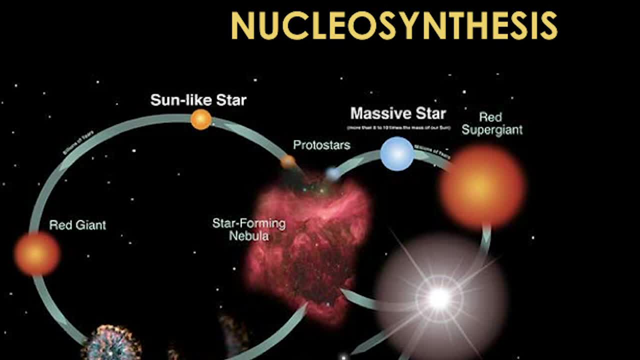 These protostars rotate faster and increase in temperature as they condense and further contract. As the protostar contracts, the central temperature increases to the point of igniting a series of nuclear reactions. This is also the beginning of the main stages of the hydrostatic stellar evolution, where stellar nucleosynthesis occurs. 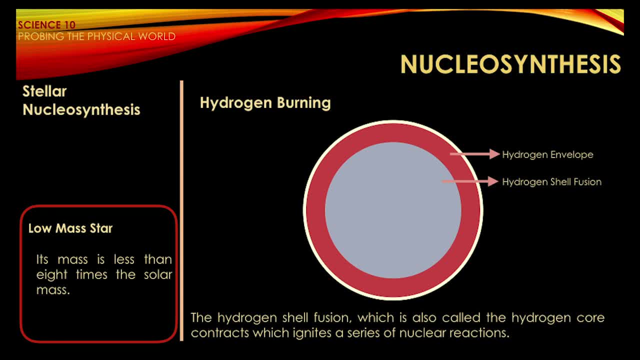 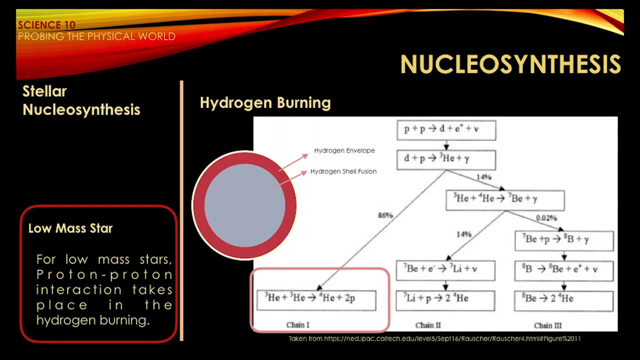 The first stage of the series of nuclear reactions is called the hydrogen burning stage, where the hydrogen core is converted to heavier elements. The nuclear reactions that happen in this stage depends on the mass of the star. If the star is a low-mass star, that means a star with mass less than 8 times our sun's mass. proton-proton interaction, or PPI, takes place in converting the hydrogen core into helium. 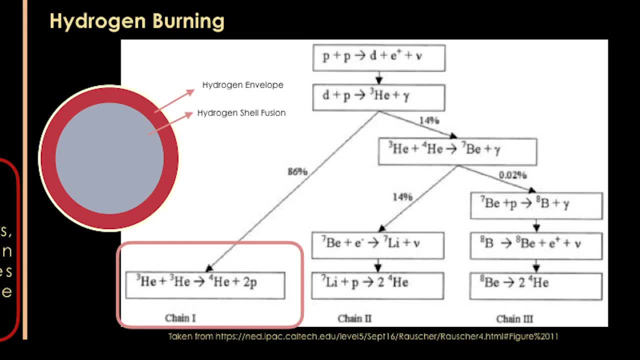 This interaction has three chains, and 84% of the nuclear reactions that occur on this type of star are in the chain 1 reaction, while the remaining percentage are in the chains 2 and 3 reactions. The PPI reaction creates a new inner core which is made of helium. 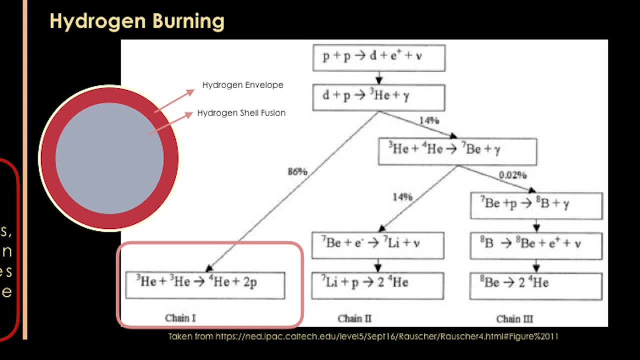 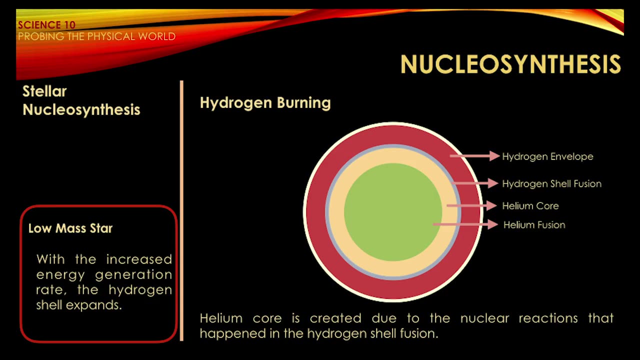 Once the hydrogen shell fusion is almost depleted, the newly formed helium core contracts, thereby increasing the inner temperature and, at the same time, increasing the energy generation rate at the hydrogen shell. With the increased energy generation rate at the hydrogen shell, this causes the star to expand enormously in luminosity and size. 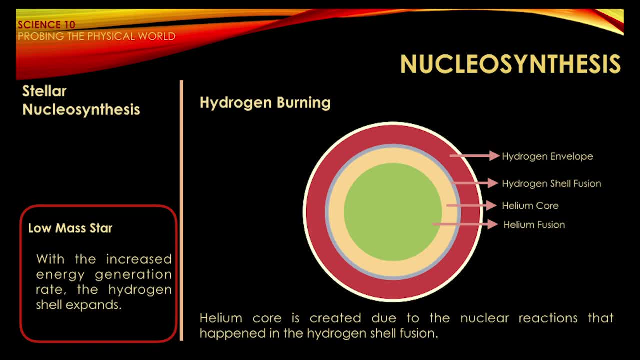 The star becomes a red giant. The contracting helium core begins another nuclear reaction. This is the helium burning stage. At this stage, the inner parts of the helium core is burned to create another core made of carbon with some specks of oxygen, via the triple alpha process. 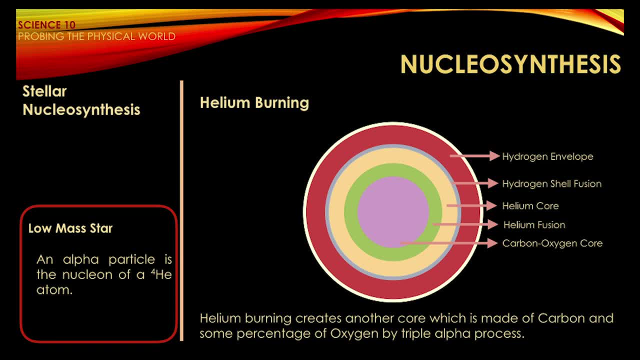 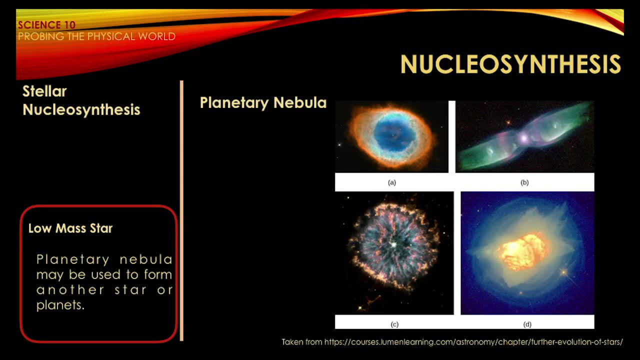 An alpha particle is the nucleon of helium-4, which is composed of two neutrons and two protons. This is the last stage of the series of nuclear reactions. As the low-mass star depletes its source of energy generation, the two outermost shells, the hydrogen and the helium shells, asynchronously contract and expand until such time these are dispersed from the star and form a planetary nebula. 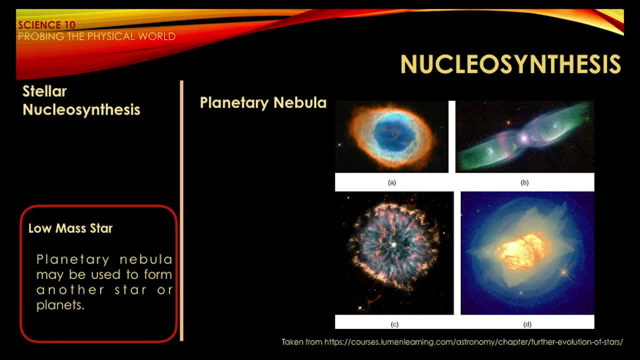 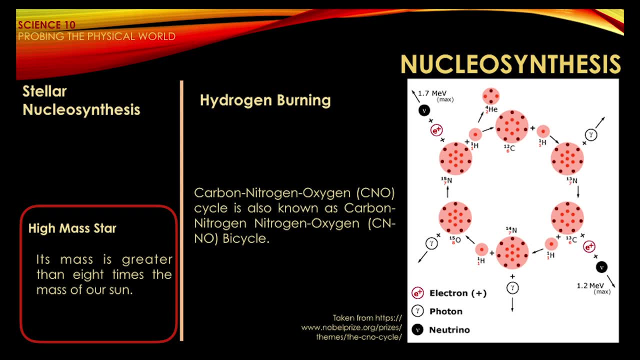 What is left is a white dwarf star, which is the last inner core created in this stellar evolution For high-energy stars. this is the last inner core created in this stellar evolution For high-mass stars, stars which have masses greater than 8 times our sun's mass. carbon-nitrogen-nitrogen-oxygen, or CNNO bicycle, also known as carbon-nitrogen-oxygen or CNNO cycle, may take place in the hydrogen burning stages. 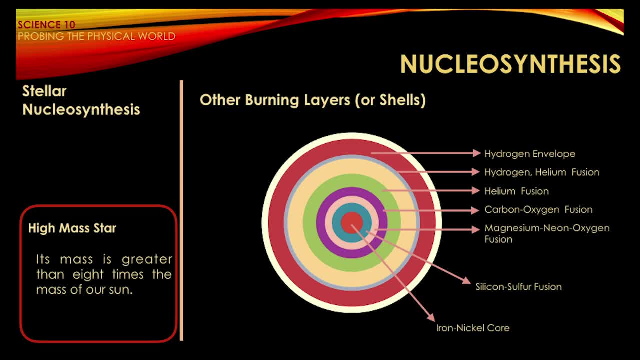 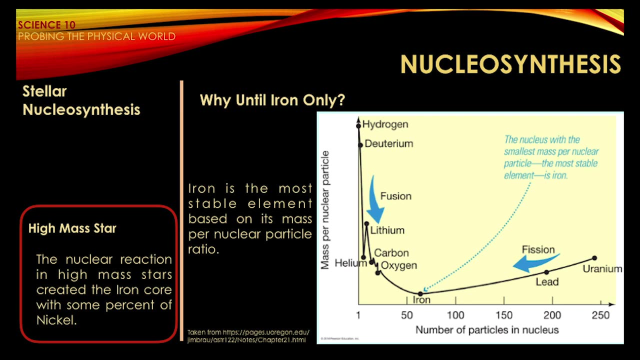 The series of nuclear reactions does not stop with carbon core on this type of star. It continues until an iron core with some percentage of nickel is made. Once an iron core is made, no further nuclear reactions will follow. It is said that iron is the most stable element, based on its mass per nuclear particle ratio, as shown in the graph. 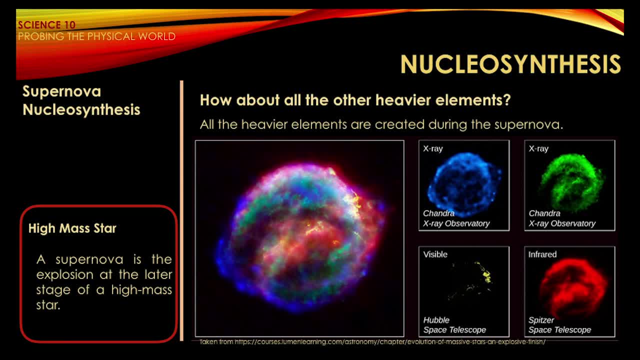 Now, how about the remaining elements? The remaining elements were created during the biggest fireworks display in the universe, the supernova. Supernovae happen when high-mass stars deplete their source of energy generation, which leads to explosive endings. In this stage of the stellar evolution, all elements were formed, but almost all were unstable, which lead them to either decay into lighter, stable elements or they cease to exist. 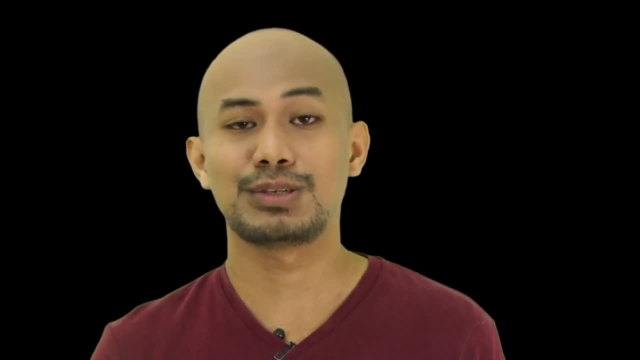 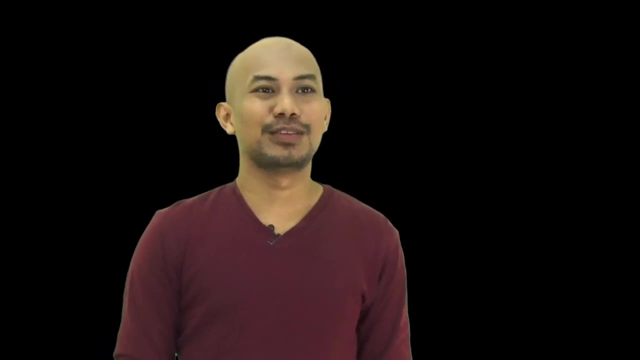 Now, what's so similar about the fireworks display in the supernova? Both of them make big explosions and spectacular colors. The main difference between the two is that the temperature and pressure is too high in the supernova that it can create spontaneous nuclear reactions to form the heavier elements.